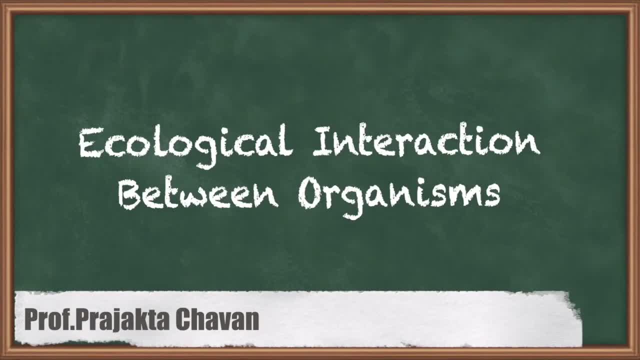 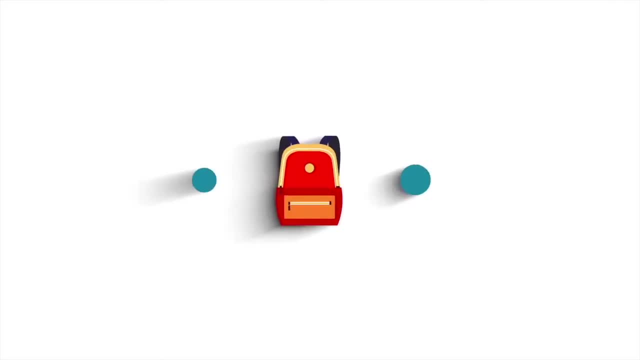 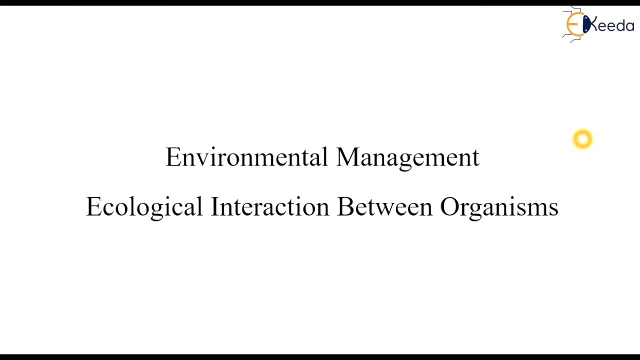 In this lecture we are going to see ecological interaction between different organisms under the subject of environmental management. This is the last part of topic ecology or concept of ecology. In previous part we have already covered what is ecosystem, what is concept of ecology. 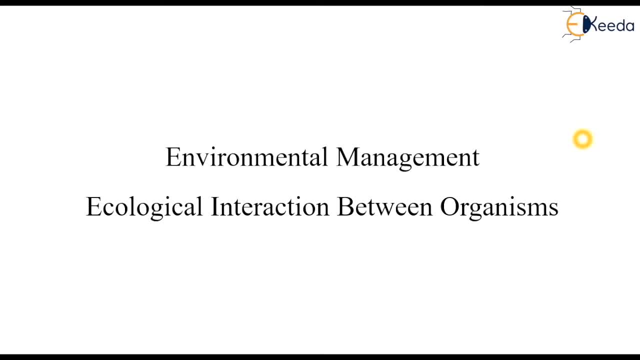 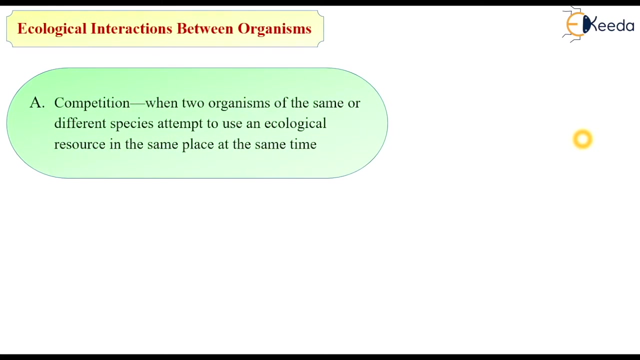 what is food chain or food web and what is ecological pyramid. So this is the last part and most important part, that is, interaction between different organisms in ecosystem. So let's we see. So what is the ecological interaction between organisms? So there are different levels or different factors on that. 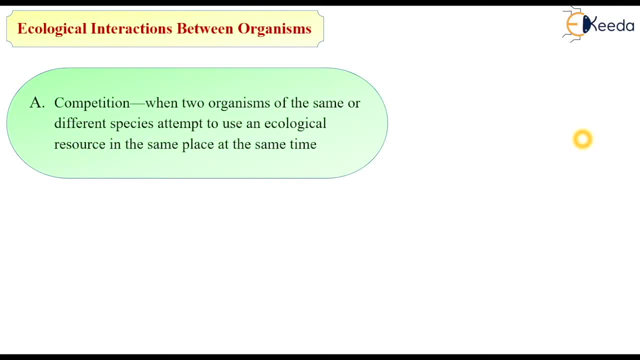 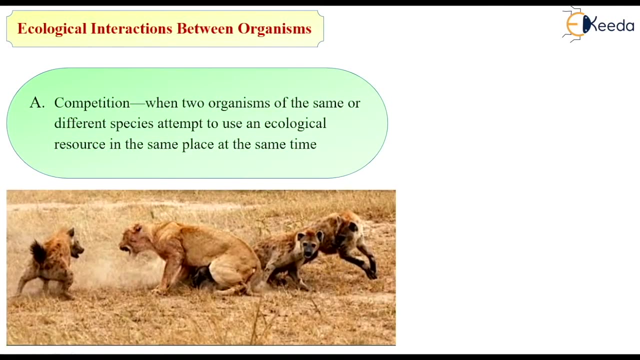 So organisms are dependent. First factor is competition, When two organisms of the same or different species attempts to use an ecological resources in the same place at the same time. As you can see in this diagram, You can see this lion and this cheetah. both the species of carnivores are different. 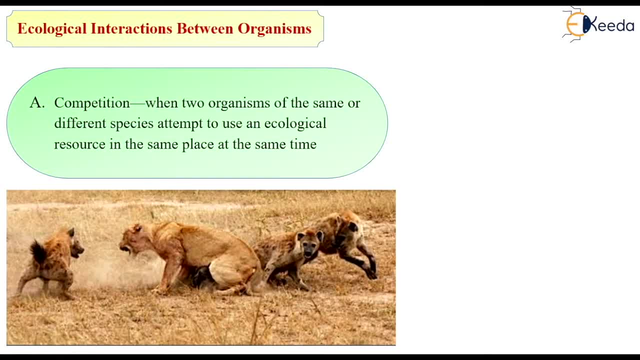 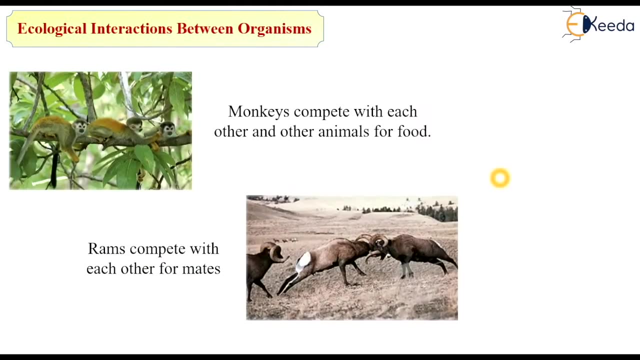 But again they are using the same natural platform of ground Or this grass for its playing game, or different reasons. So they are using a single environment, But the species of organisms are different. Again, as you can see in this first diagram, that is, monkeys compete with each other and other animals for food. 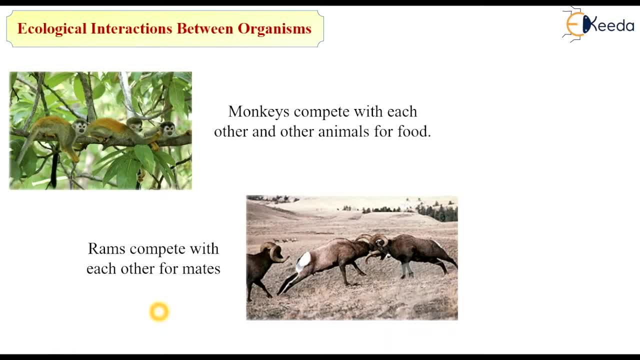 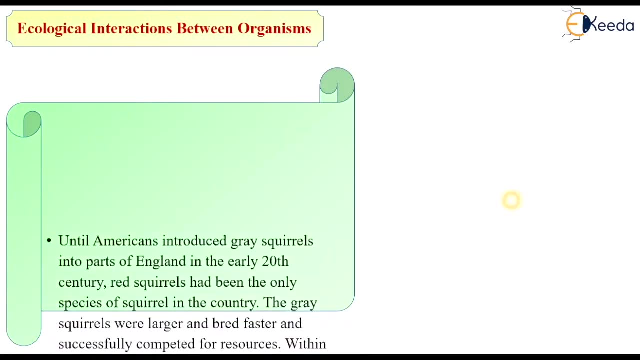 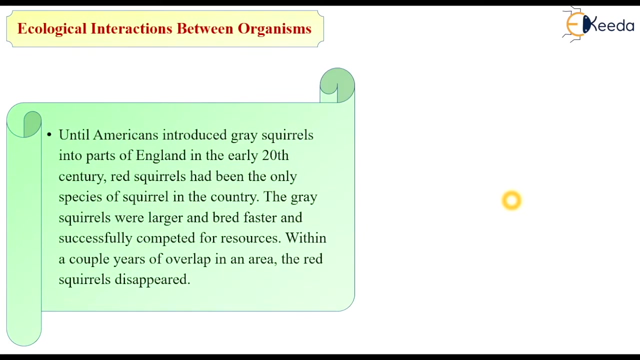 Also- this is the next example- that rams compete with each other for mates. So this is the factor of competition between the different organisms, and for that they are using the same platform of environment. So until the Americans introduced grey squirrel into part of England in the early 20th century, red squirrels had been the only species of squirrel in country. 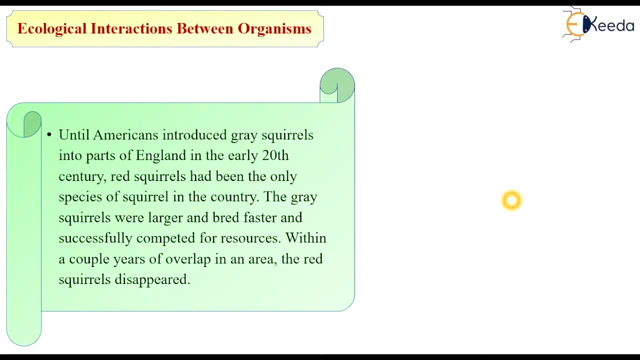 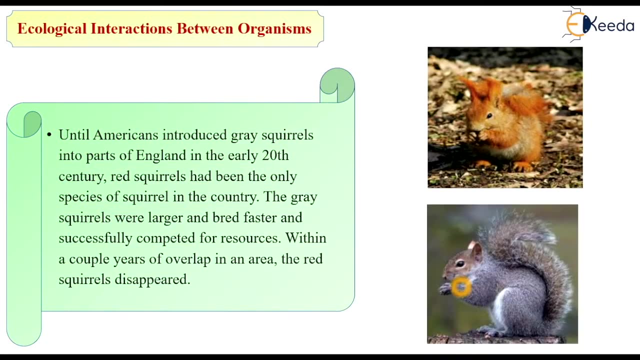 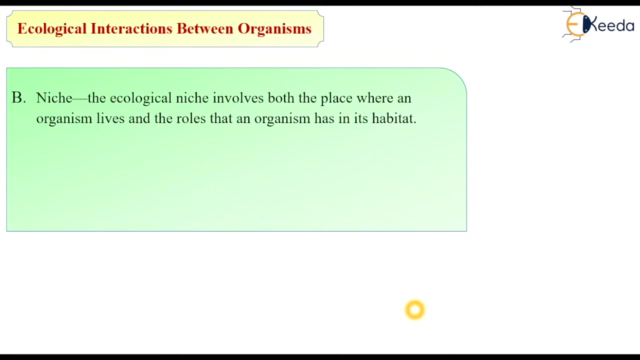 The grey squirrel were larger and breed faster and successfully competed for resources. Within a couple of year of over life in an area, the red squirrel disappeared. So this is the image of red squirrel And this is grey squirrel Again. Nike- that means the ecological Nike involves both the places where an organism lives. 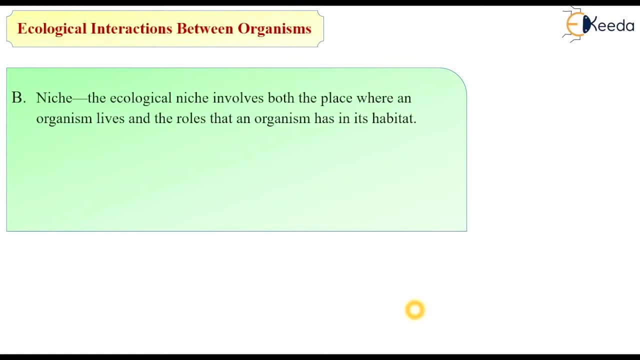 And the role that an organism has in its habit- For example, the ecological Nike of a sunflower growing in the background- include absorbing light, water and nutrients for photosynthesis, Providing a shelter and food for other organisms, for example bees, ants, etc. 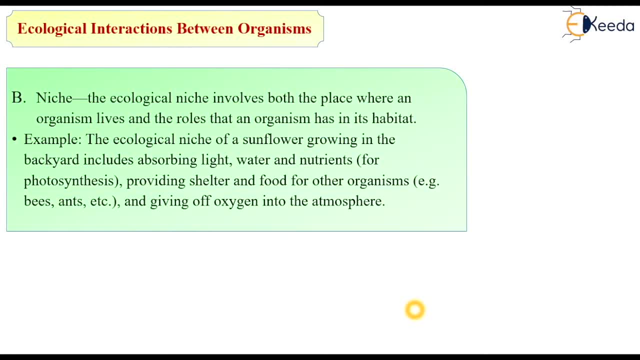 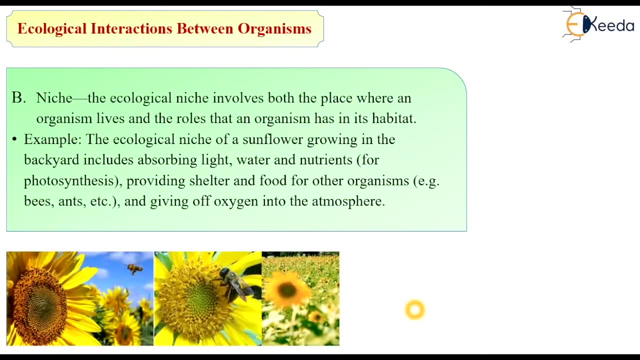 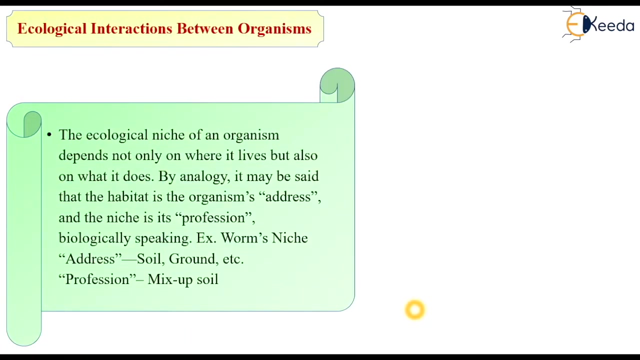 So both the organisms are dependent on each other And giving of oxygen into the atmosphere. So these are the set of organisms, or set of factors or parameters Which are act a both the roles, that is, producers as well as consumers. Again, the ecological Nike of an organism depends on only on where it lives, but also on what it does. 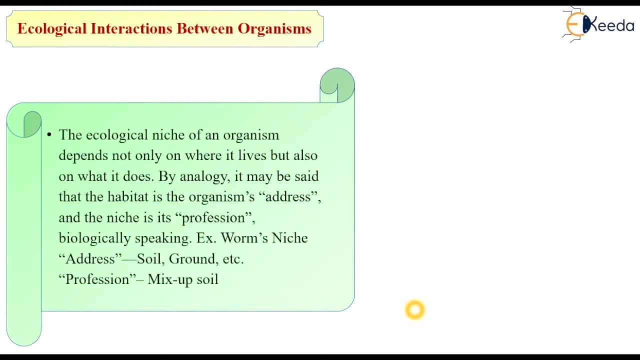 That means, by analogy, it may be said that the habitat is the organisms address and Nike is the its professions. Biologically speaking, for example, worms, Nike addresses soil, ground etc. and by professional, it mix with up a soil. So, as you can see in this diagrammatic representation, 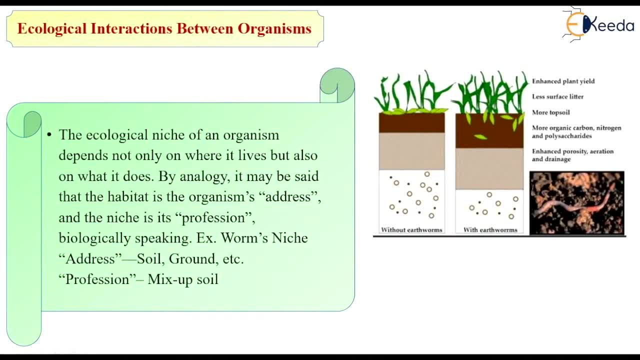 So earthworms are using the environment, The environmental source, as soil and the without earthworm and this is the with earthworm. So, again, by using earthworm, the producers, the energy getting to the producers are increasing, So that by the production of this, producers are increasing. 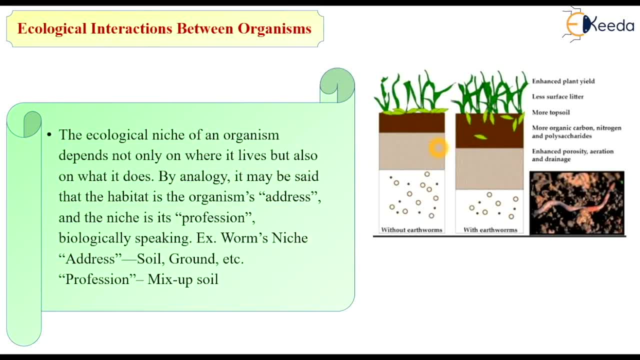 But without earthworm. only by using the soil as a source of energy, the plant growth is reducing. So by using the earthworm it will enhance the plant till, less surface litter, more topsoil, more organic carbon, nitrogen and polysaccharide and enhance the porosity, aeration and drainage. 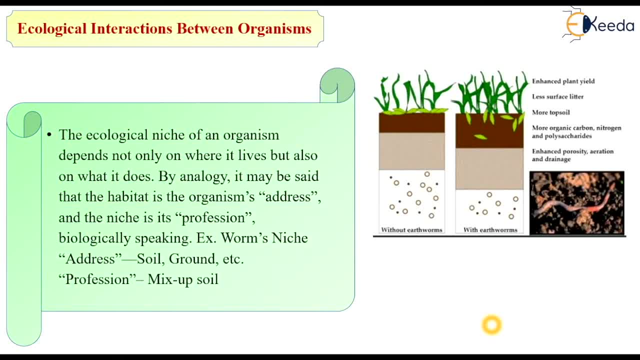 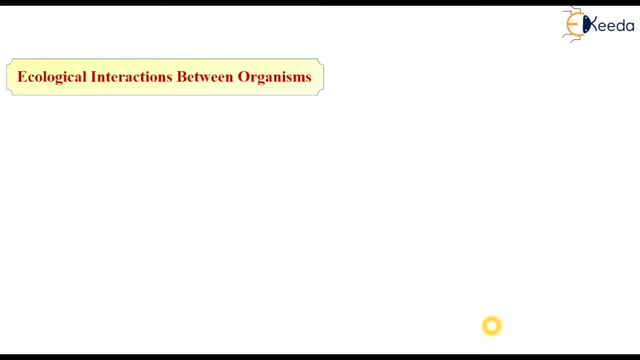 That means the non-living and living organisms are. there are the interaction between these organisms and they are dependent on each other. Next is predation. In this state, the one organism capture and feeds an another organism. Next, the first is predators, that is, one that does the killing. 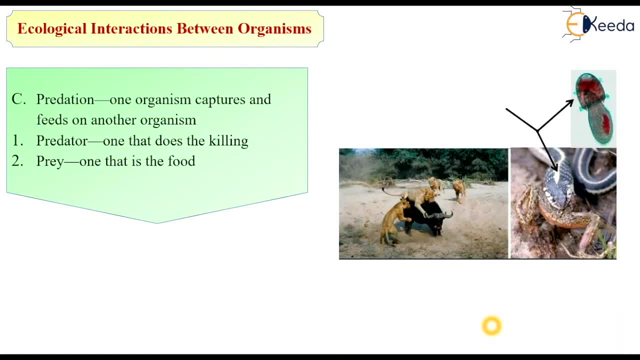 Second is prey, that one that is a fool, As you can see in this example. So one is predator, that one that does the killing, So this line is predator. And second, one is prey, that is one that is a fool, So that frog or other organism is the fool for this killing animals. 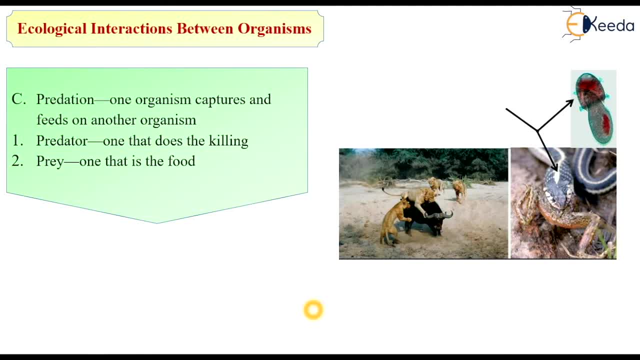 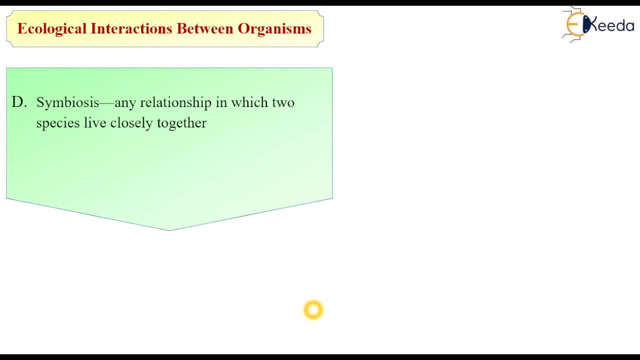 So the overall combination is called as combination of predator and prey is called as predation. The fourth level is symbiosis. That means any relationship in which two species lives closely together, For example mutualism. Both the species benefits, win-win condition. 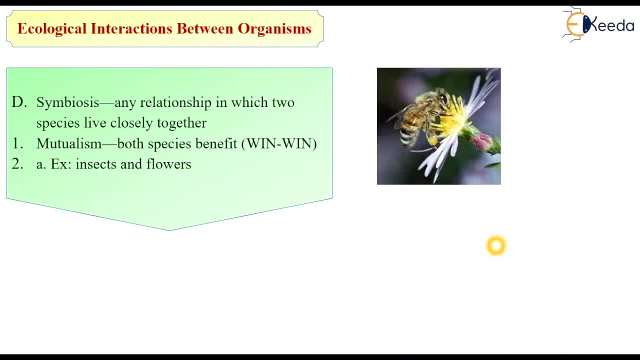 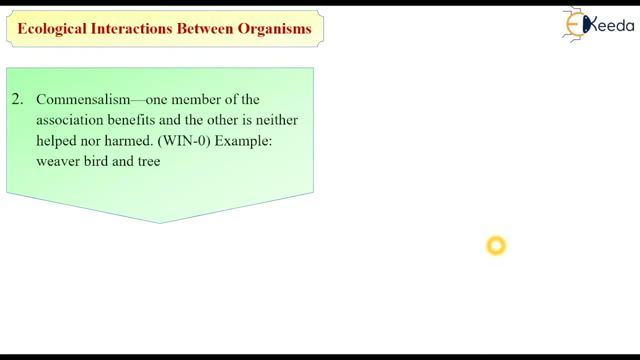 For example, insects and flower. So both are dependent on each other. That are the symbiosis. Next one is commensalism, That is, one member of the association benefits and the other is the neither help nor harm, For example, weaver birds and tree. 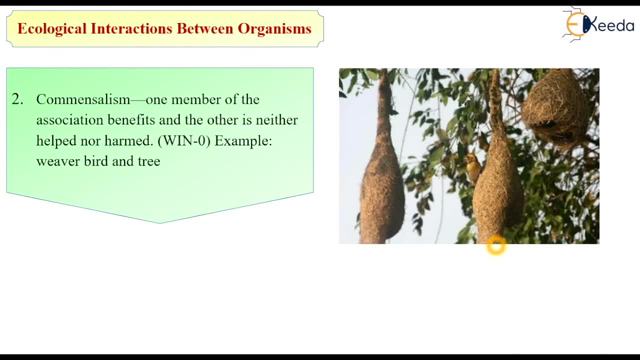 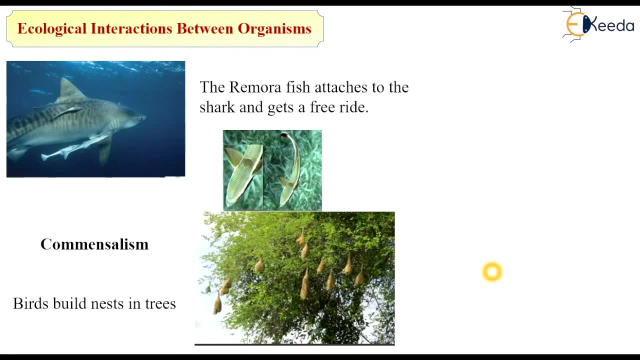 So both are the beneficial and not harm for the each other. So examples of commensalisms are, As you can see in this diagram, The remora fish attacks to the shark and get a free ride. So again, these are not harmful to each other. 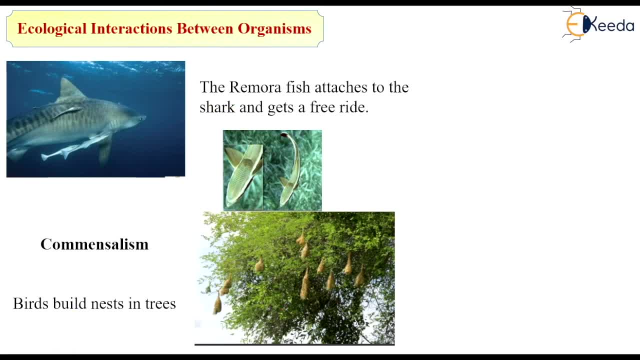 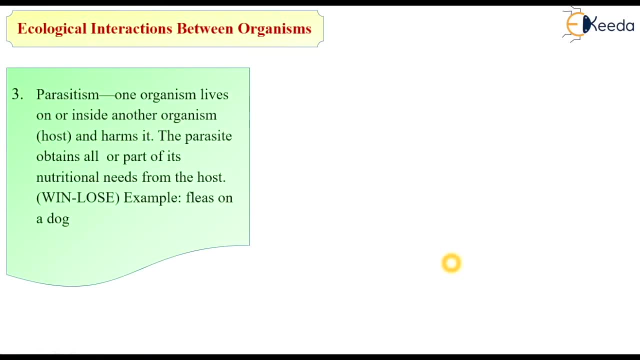 And next example is bird build a nest in treads. So both are beneficial to each other and dependent on each other without getting any harm. Next is parasitism, That are the one organism lives on or inside another organism In form of host and harms it.